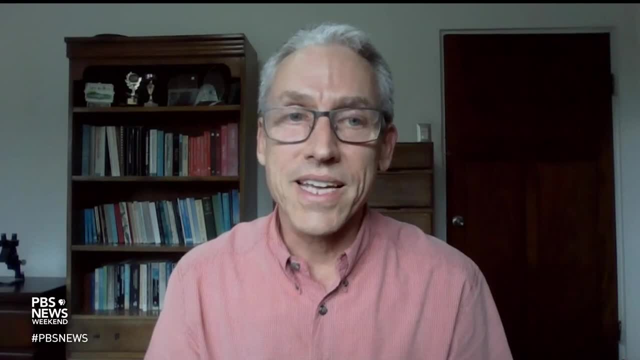 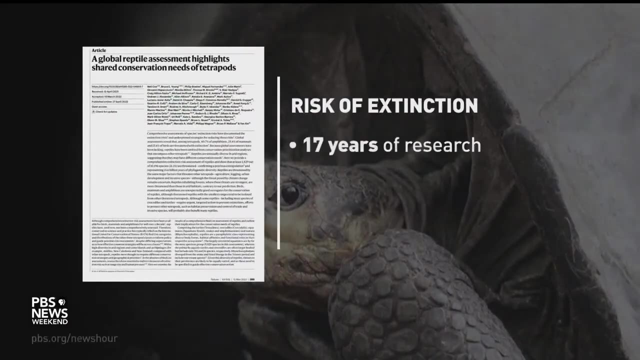 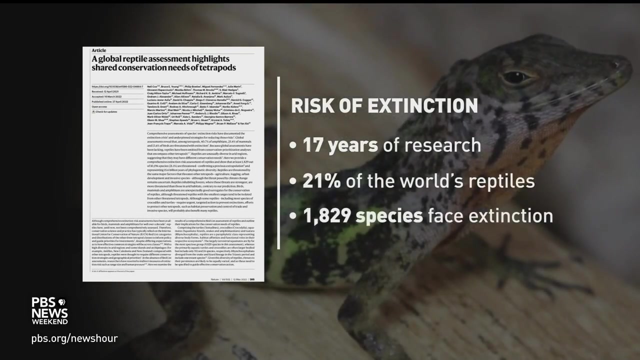 known. at the time We worked with over 900 scientists from around the world that did know these species. Young says the research took 17 years to complete and found that at least 21 percent of the world's reptiles- more than 1,800 species in all- face extinction. Why are so many reptiles in danger of extinction? BRUCE YOUNG, ZOOOLOGIST, KOMODO, DRAGON. There's a few reasons why most reptiles that are endangered are in fact endangered loss of habitat, especially forest habitat. from logging. Also, the expansion of the agricultural frontier has caused many habitats for reptiles to die. BRUCE YOUNG ZOOOLOGIST KOMODO DRAGON. The study also found that if all threatened reptiles were to disappear, the world would lose a combined 15 billion years of evolutionary. 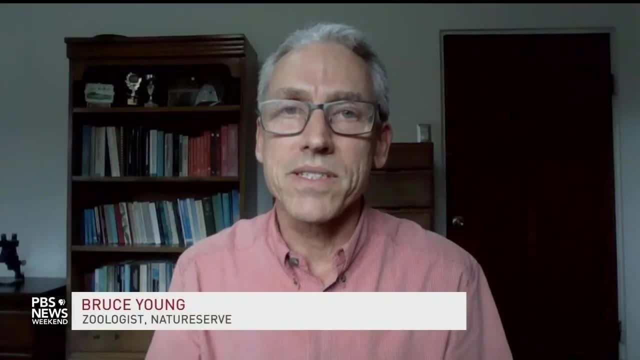 history. BRUCE YOUNG ZOOOLOGIST KOMODO DRAGON. It will take a big contribution by governments to kind of change the trajectory we're on. BRUCE YOUNG ZOOOLOGIST KOMODO DRAGON. One of the reptiles most at risk: Turtles. 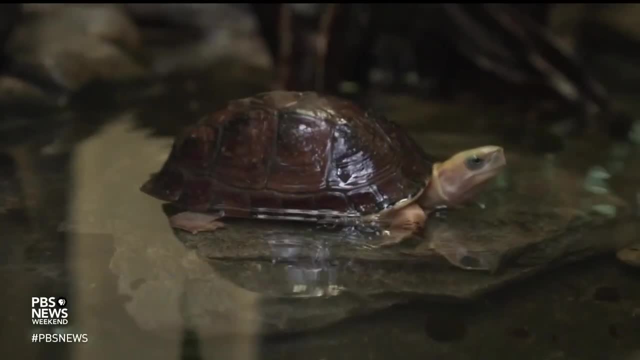 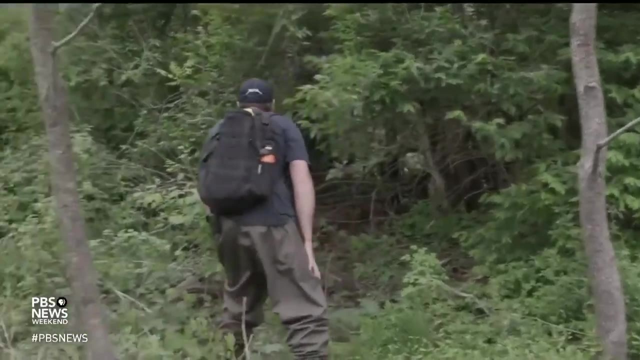 with nearly 60 percent of the species facing extinction and in need of targeted conservation efforts. BRUCE YOUNG ZOOOLOGIST, KOMODO DRAGON. We're surveying both the land and the stream, hoping to find some turtles. 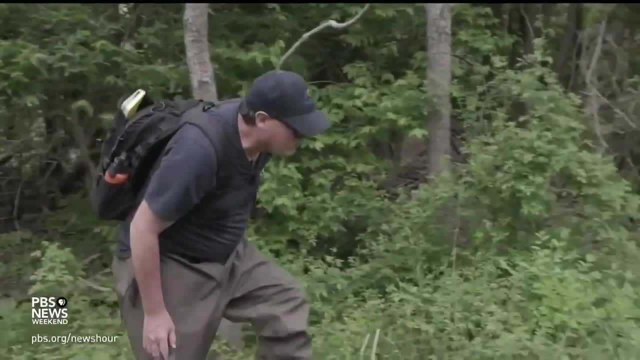 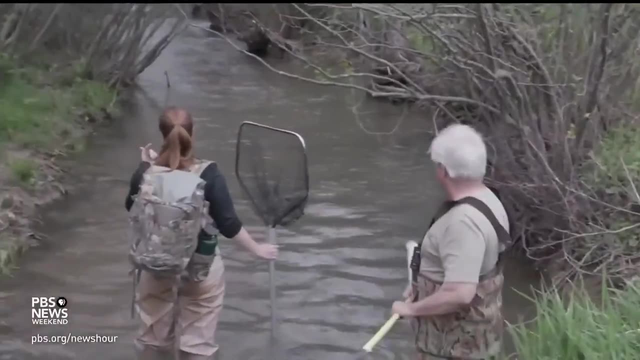 SCOTT SMITH IS A WILDLIFE ECOLOGIST FOR THE MARYLAND DEPARTMENT OF NATURAL RESOURCES. HE'S BEEN STUDYING THESE SLOW-MOVING REPTILES FOR 30 YEARS. SCOTT SMITH, MD, MD, MD. Okay, everybody ready. 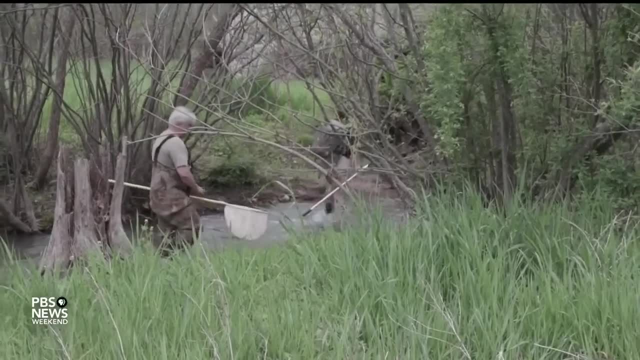 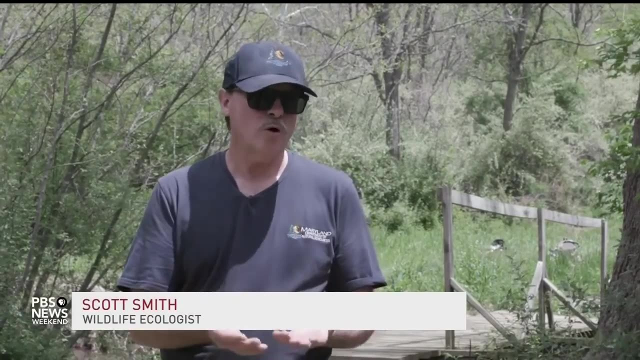 We tagged along as he and a team of scientists surveyed wood turtles in Western Maryland, SCOTT SMITH, MD, MD. MD. Wood turtles' main threats are habitat losses, road kill, road mortality, collecting for the pet trade, climate change. And we wouldn't know that. 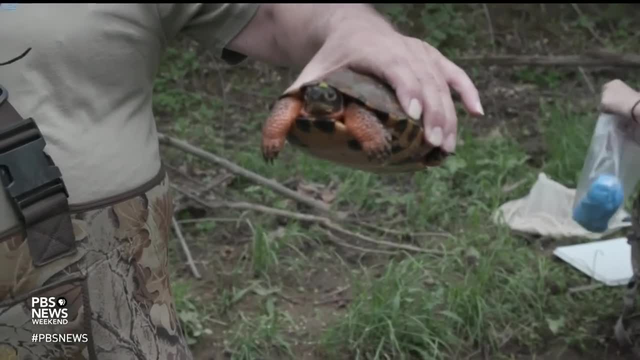 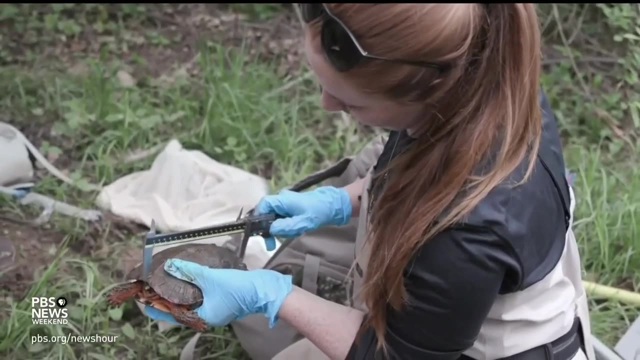 basic stuff without having come out and seen it. BRUCE YOUNG, ZOOOLOGIST, KOMODO DRAGON. We've come out and done these surveys, 71 for shell, height 71.0,. okay, SCOTT SMITH, MD, MD, MD. These scientists mark and measure each turtle they find. 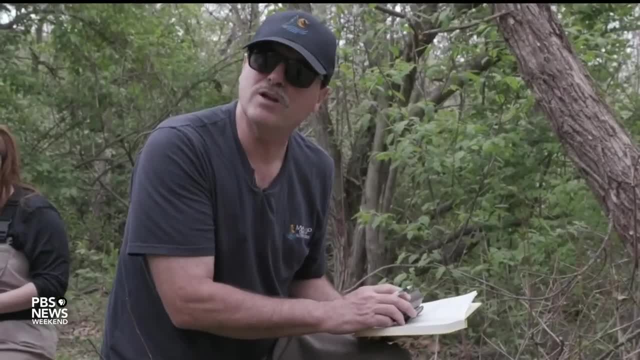 One problem we're having here is with reproduction. We have not found any youngsters at all. SCOTT, SMITH, MD, MD. And Smith says nearly all of the turtles they are finding are females. Female, What do you got? 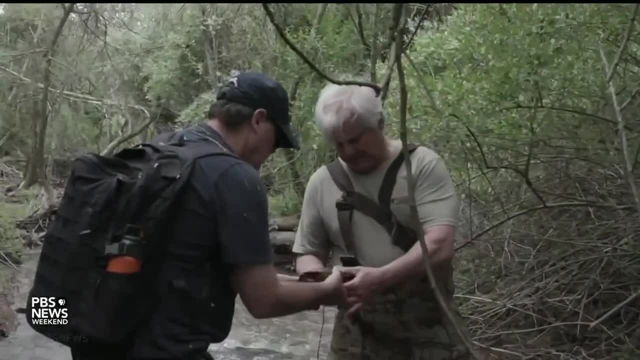 Probably female. SCOTT SMITH, MD, MD, MD. We're seeing skewed sex ratios towards females because of higher incubation temperatures due to climate change And, of course, in nature. you want a 50-50 situation. 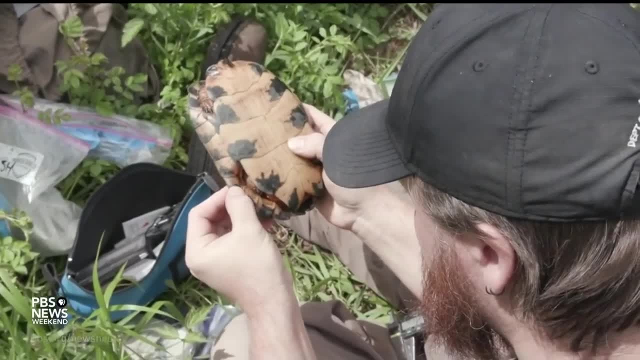 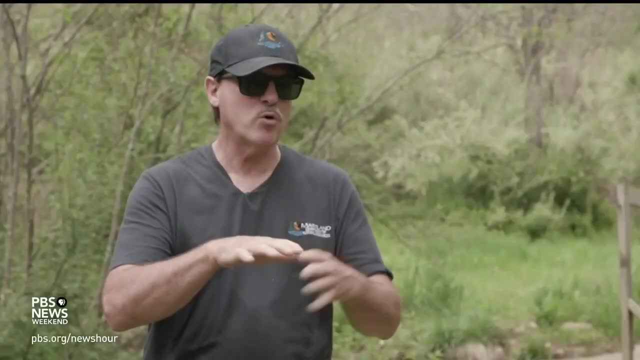 SCOTT SMITH, MD, MD, MD. Another major issue: human development in areas turtles have long called home, leading to an increase in predators like raccoons. SCOTT SMITH, MD, MD, MD. There's a lot more in the landscape now than there were. 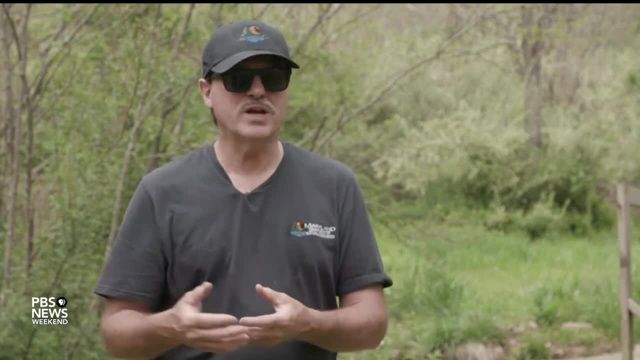 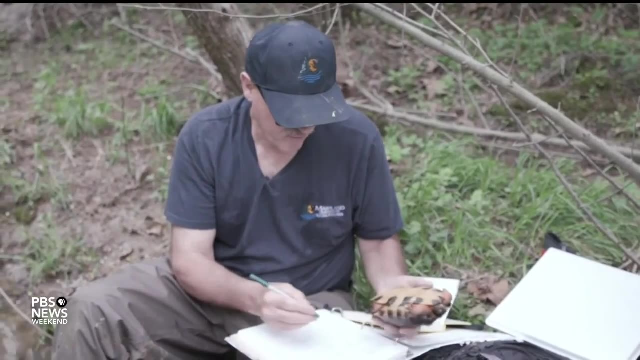 historically, because they can feed off our garbage. They can feed off cat food, dog food we leave out, And so we have these absurdly elevated populations of predators which feed on turtle nests. SCOTT, SMITH, MD, MD, MD. And while these reptiles face a host of threats, Smith says, 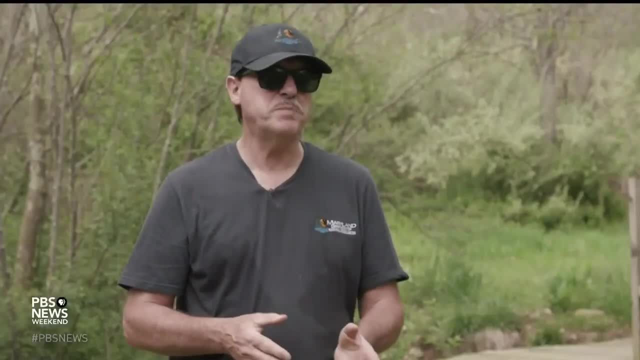 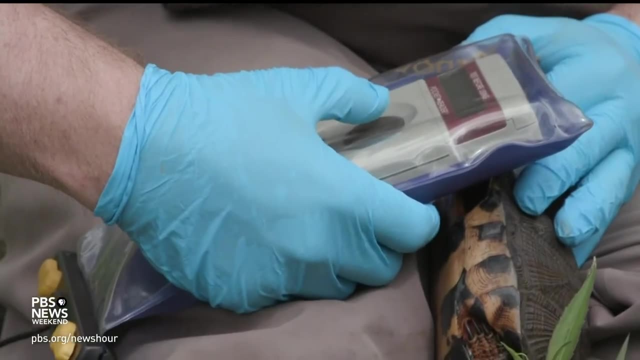 turtles around the globe are the biggest predators. SCOTT, SMITH, MD, MD, MD, MD. Certain species are really on their last legs before they go extinct. So we certainly have a lot of problems, But comparatively to most of 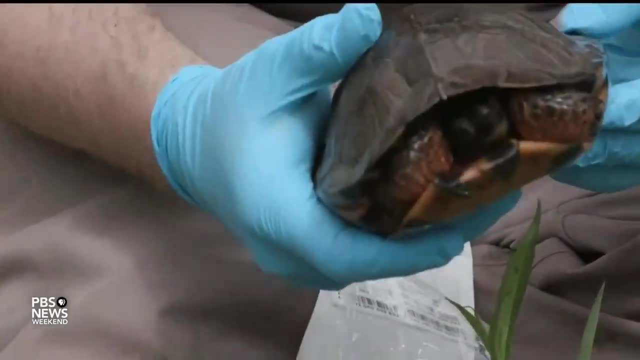 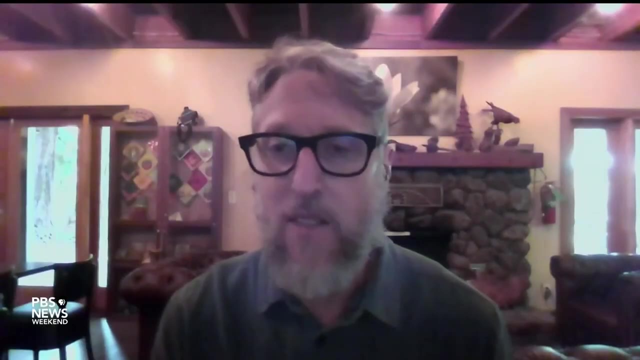 the rest of the world, our turtle populations are doing relatively well. NOAH GREENWALD, MD. Turtles actually survived the meteor that killed the dinosaurs. So you know they survived a giant asteroid hitting the planet, but they might not survive us. 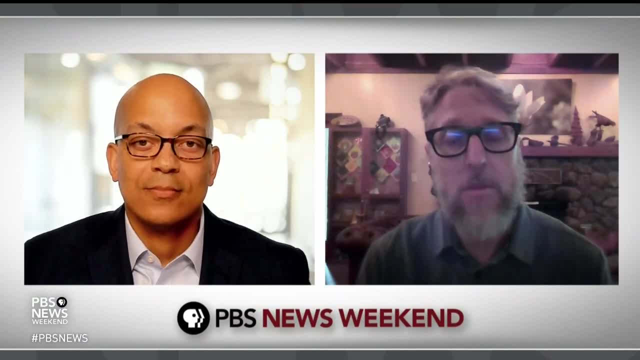 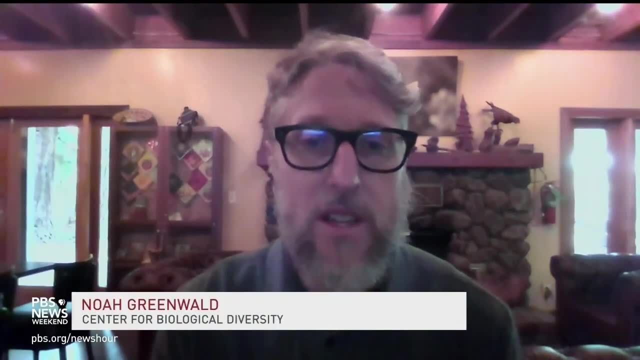 SCOTT SMITH, MD. MD. MD. Noah Greenwald is the endangered species director at the Center for Biological Diversity. NOAH GREENWALD, MD. MD. Many reptiles control small mammal populations. They control. 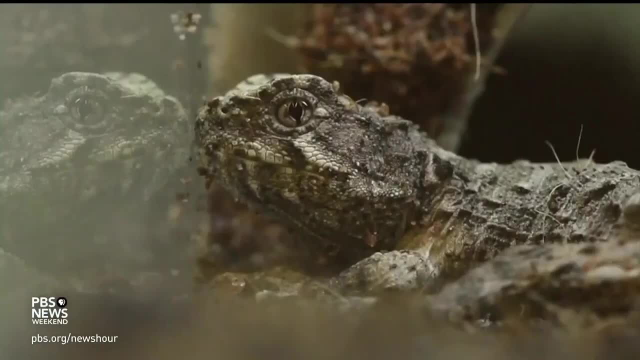 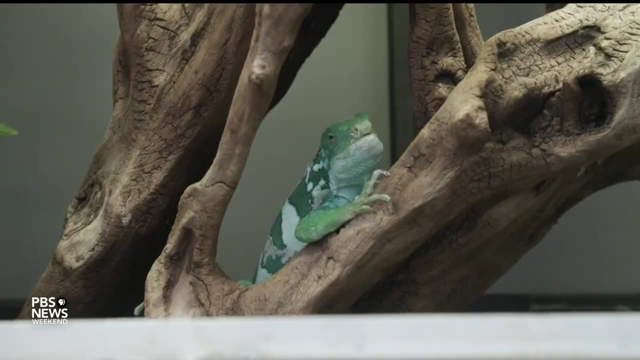 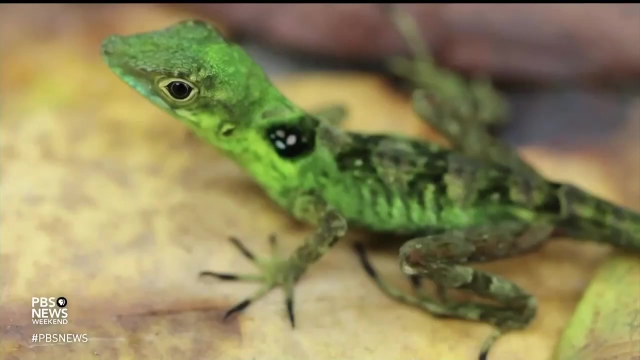 insects, which then has impacts elsewhere in the ecosystem. You know those insects, then don't eat plants and don't otherwise affect things. One of the concerns about losing biodiversity is that you know. nearly all of our medicines, all of our foods come from species. So as we lose these species, you know we potentially 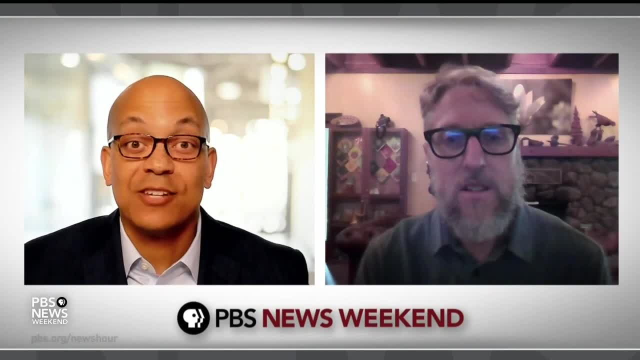 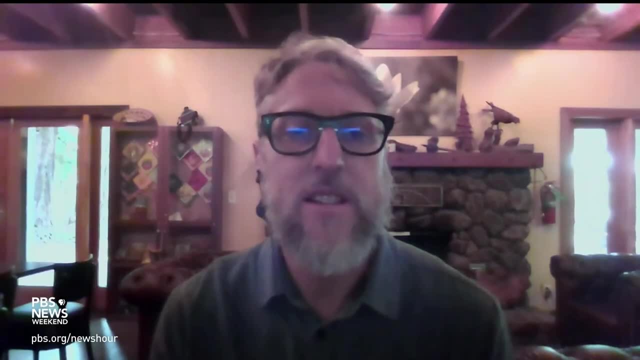 lose a cure to cancer. GEOFF BENNETT MD. So what's the solution, then, to the extinction crisis? NOAH GREENWALD MD. A lot of the solution to the extinction crisis is actually also a solution to climate change, that these two problems are quite interrelated And, in particular, 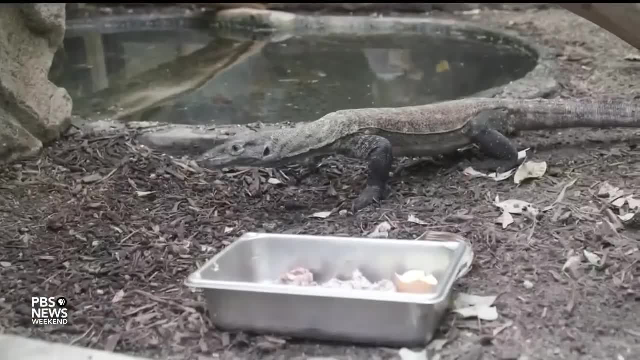 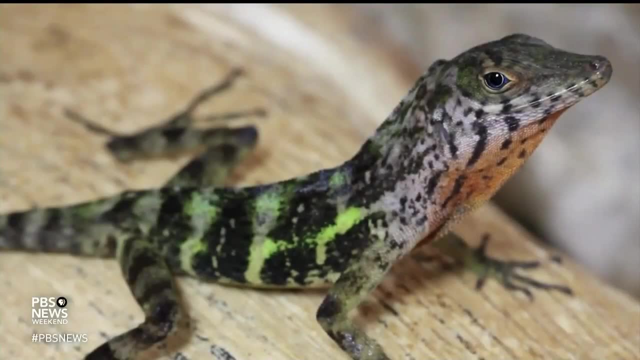 we just have to protect more of the natural world so species have space to live. GEOFF BENNETT, MD. While threats to reptiles have become increasingly urgent, wildlife ecologist Scott Smith says there's still time to act. SCOTT SMITH, MD. Thank you. 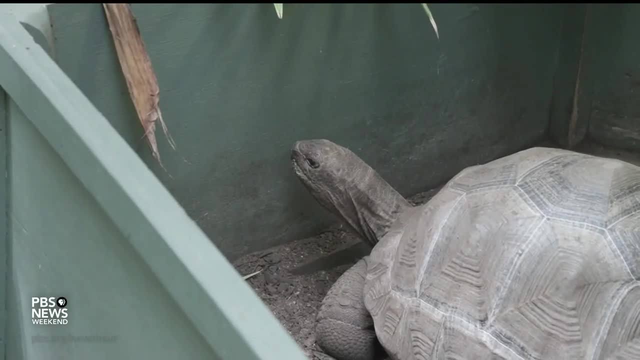 GEOFF BENNETT MD. It's not all bad news. We as humans can certainly change our behaviors and act to reverse this trend, but we have to do it now.